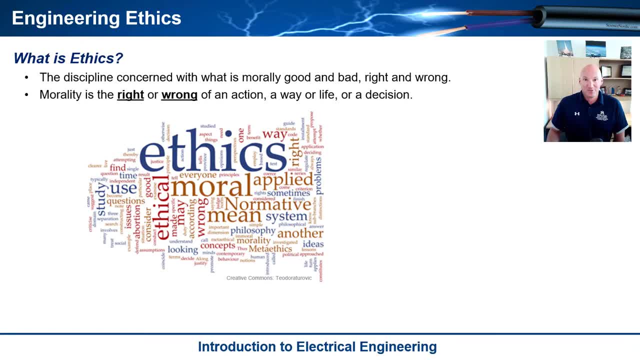 not something that an electrical engineer is going to try to contribute to, But what we want to do is we want to try to take what these, what ethicists and philosophers, philosophers have, you know- basically come up with and try to help guide our engineering. 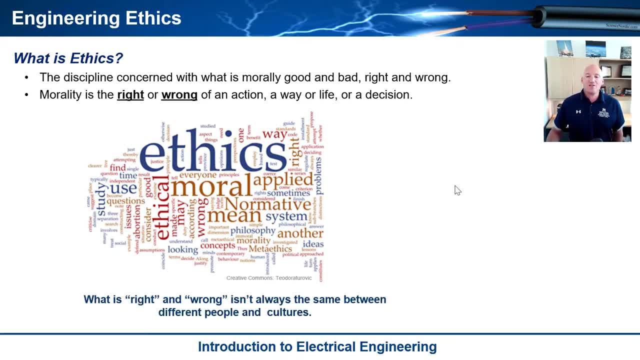 decisions, okay. So what makes it really challenging is that what people think is right or wrong isn't always the same. okay, It's not. you know, laws are easy right. Laws are: you break the law, that's wrong. But we're talking about things that aren't illegal. They're just basically decisions. 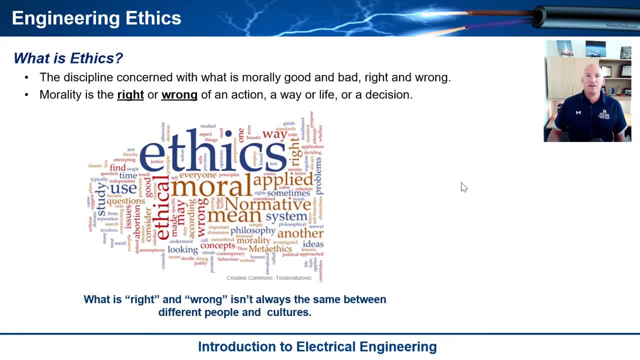 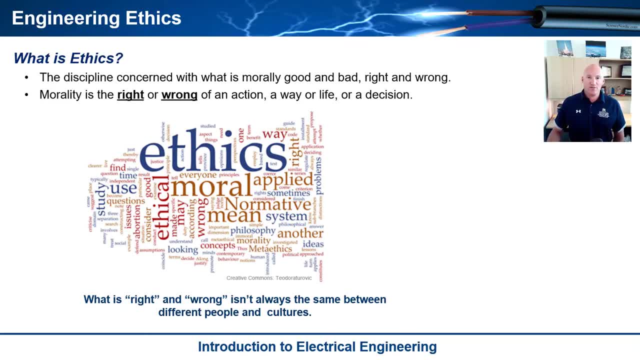 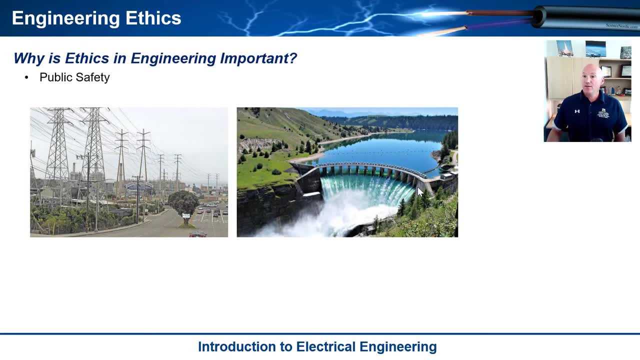 culture that you're from, So it isn't as cut and dry as you might think when you start thinking about right and wrong. Okay, so why is ethics important in engineering? Quite frankly, public safety, okay, So that's first and foremost what we need to take care of. We can, we are building. 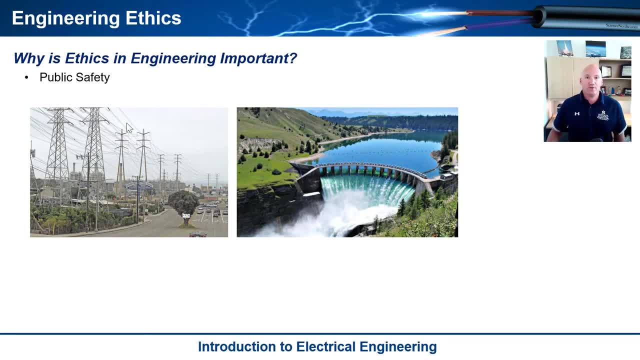 systems that are huge. okay, You think about the electrical grid. This has the capability to kill dams. I mean, think about a dam. I mean think about how amazing it is that you can hold back so much water. And if you don't make that, you know if you cut corners and make unethical decisions. 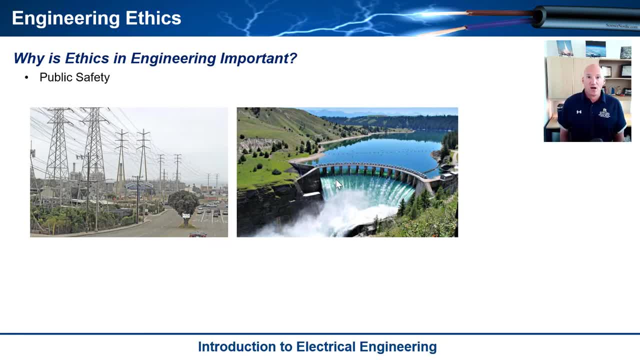 that might put profit over safety. you can see that you can cause a lot of harm to people And you know so. public safety is paramount in this. But engineering ethics today transcends that a little bit. You know public safety is number one, right, But number two- we start seeing that some. 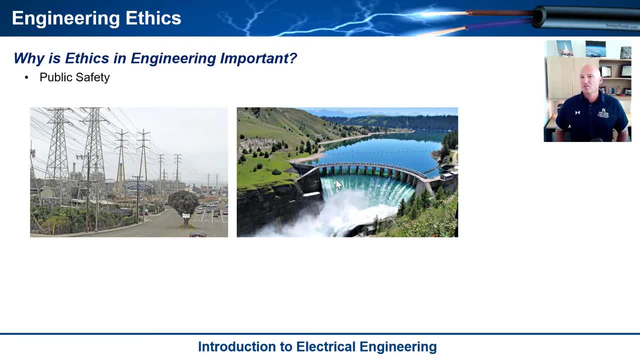 of the decisions that engineers make can kind of skew solutions that might work better for certain parts of our society compared to other parts, And so today we talk a lot about, you know, these kind of these decisions and how we might have some sort 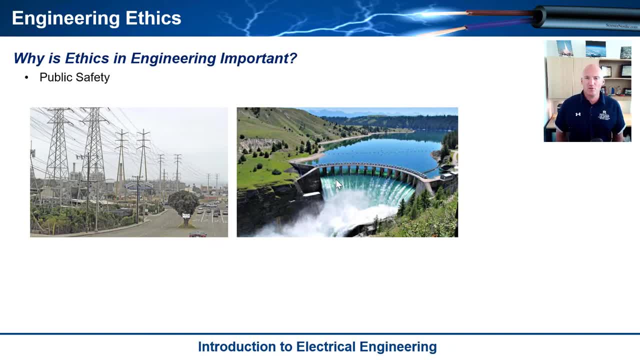 of bias toward you know our particular view of the world, And so what engineers have to do today is they really have to start thinking about society as a whole and start thinking about all the citizens within a society and thinking about you know, how do we make sure that we don't kind? 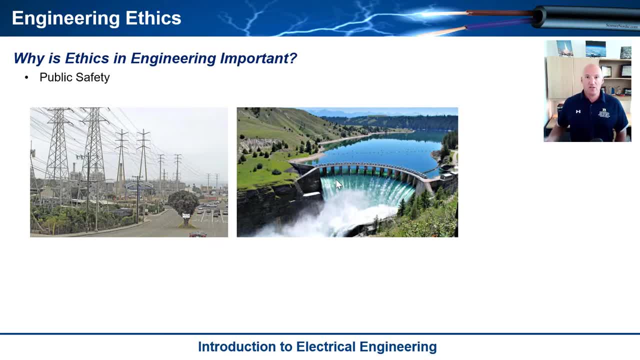 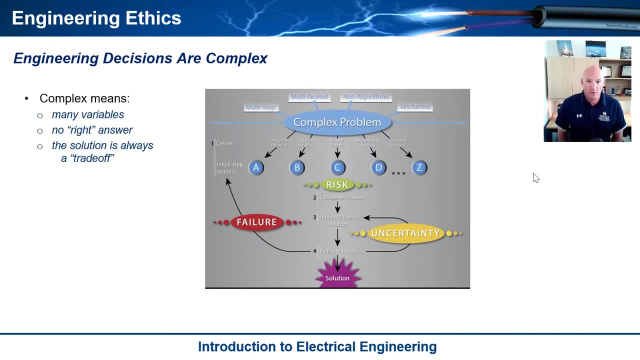 of take one part of society from actually benefiting from that to the advantage of another part. So public safety and also just kind of the whole comprehensive contribution to society as a whole. Okay, now let's think about how ethics influence our engineering decisions, First and foremost. 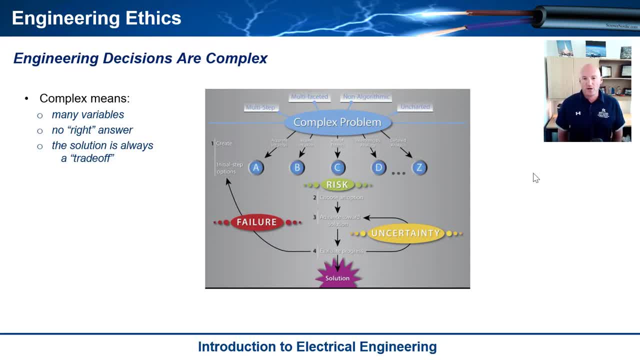 engineering decisions are complex. And so you say, well, yeah, of course they're complex, It's engineering's hard. Well, if you really think about what complex means, there is actually definition to it. So in engineering, a complex problem has to be solved, And so engineering has to. 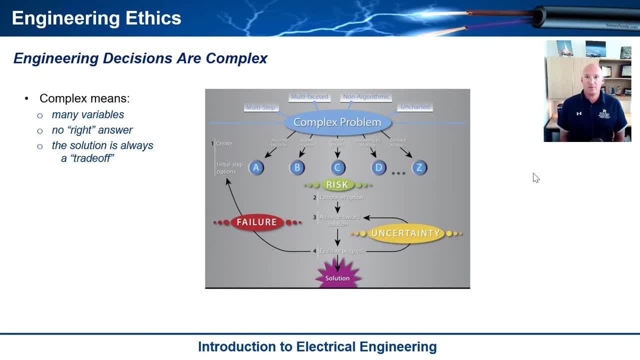 be solved as many variables. Okay, it's not just: y equals mx plus b. I mean you're talking about many, many variables that change with time and change with space and change with a lot of different factors. But what really categorizes engineering decisions today is that there's 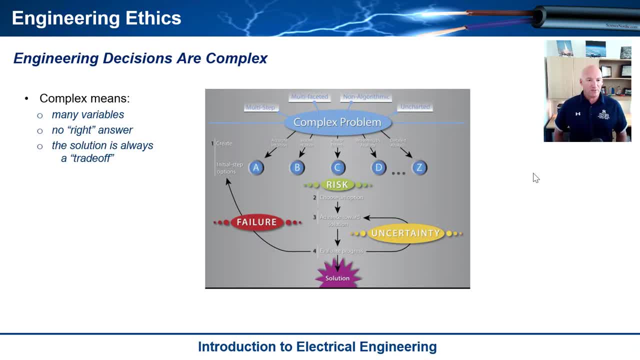 usually no right answer anymore. Okay, you know, we learn, we learn engineering problems like we solve a circuit and there's an answer. But when you go to, like, build a system, what happens is that you notice that there isn't like a solutions manual. okay, it is always a. 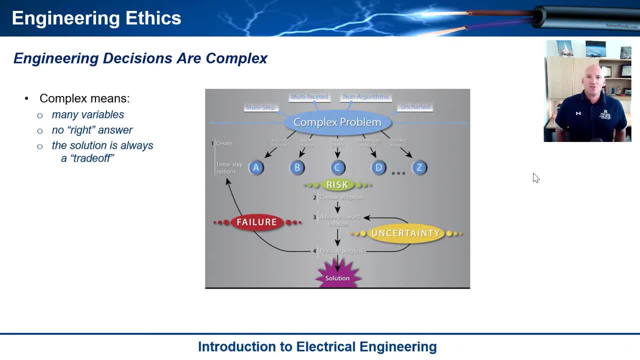 transition, And so when you go to, like, build a system, what happens is that you notice that there's a lot of different variables And you can think about it, as there's a lot of right answers to get to the end, So you can have a lot of different designs and create a lot of different. 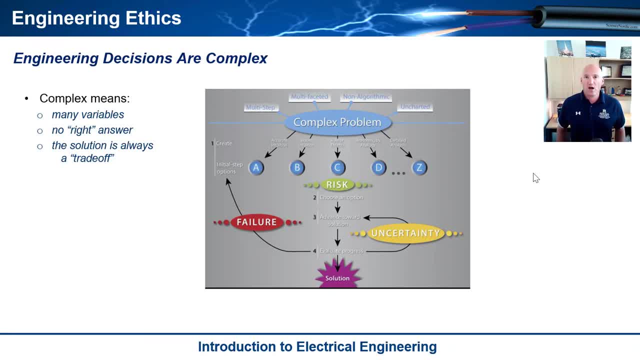 systems that actually achieve what you're able to accomplish, And so what you're really trying to do is trade off these things to try to find the optimal solution, And optimal might mean different things to different folks, So that's why engineering decisions are what we call complex. 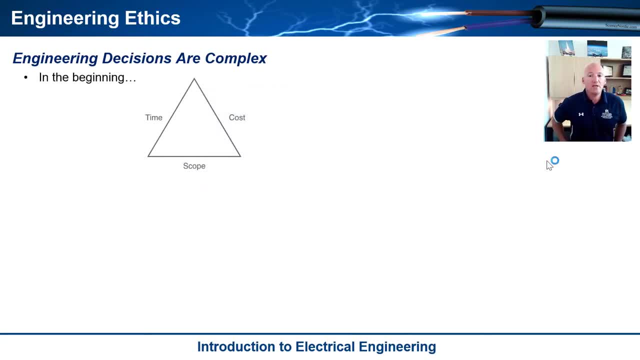 And today's problems are even more complex. So in the beginning, when you started thinking about, you know, engineering solutions, there was this thing called the engineering management or print pyramid, or design pyramid, And there were three variables that you would have. you'd have the scope, which basically means the functions of 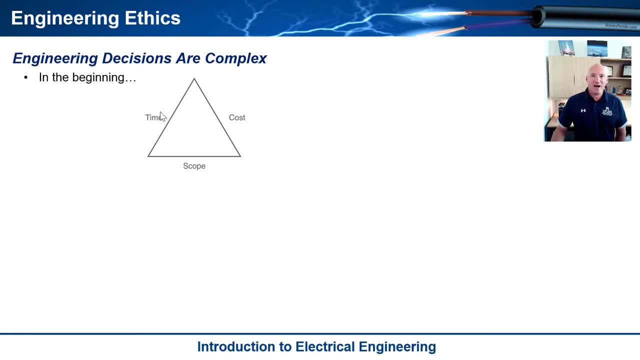 the system. So what is this system actually going to do? And then you had time and you had cost and you traded these off against each other. So, for example, if you had a new phone and it had every feature you could ever think of, it might take 10 years to develop and cost. 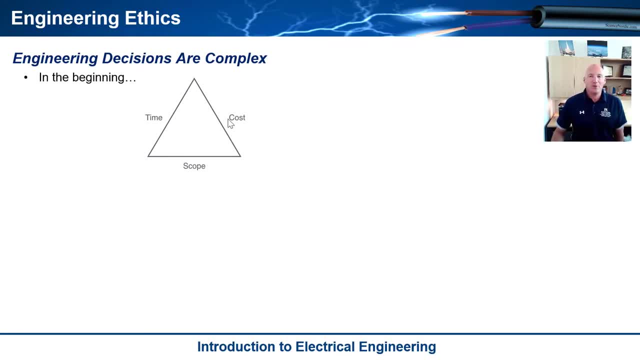 you know, and each one would cost $10,000.. So you would go: well, we can't take that long to develop, we can't have it cost that much. So we'll de-scope it, So we'll remove features until the. 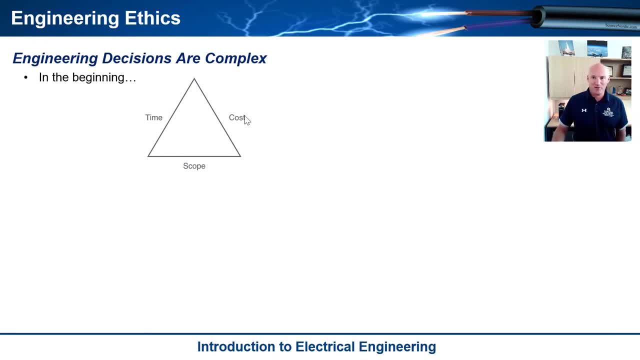 schedule gets in line with what we want and the cost gets to where we want. And then if somebody adds a feature to it, then you add time to the schedule and cost to it, And so this is kind of the standard way that engineers were trained. You know, that's how I was trained. Now, you think 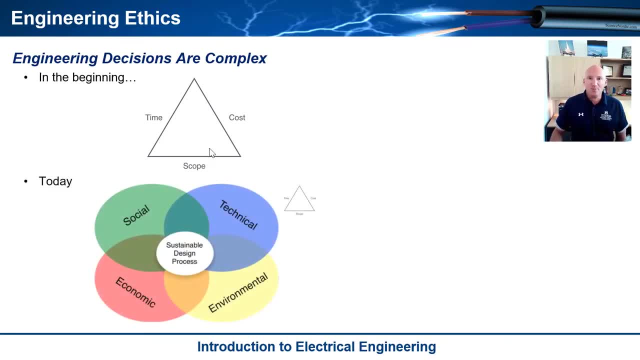 about today. it's like holy cow. So that design pyramid or project management pyramid fits within technical constraint And if you think about all the other things that engineers have to deal with today, are you have to make sure that the system that you're designing has, or you have to look at 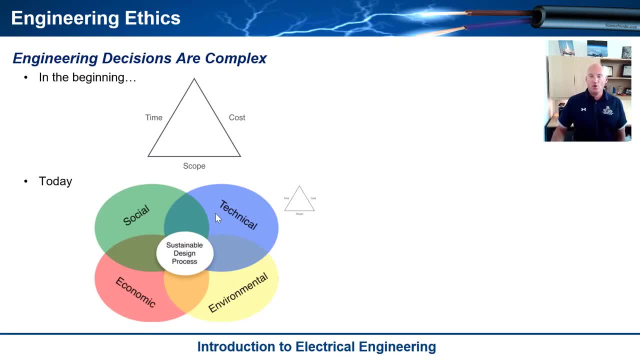 the societal impact of it. So your goal is to benefit society, right? So you got to make sure that you don't take away benefit from society or harm society. And this goes back to the whole thing of trying to design systems that benefit every citizen and not just a subset of the 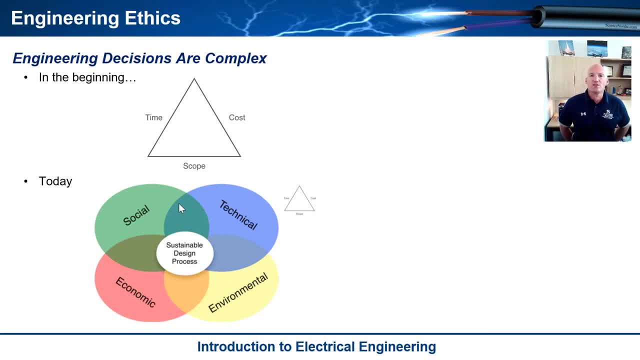 systems, And so societal impact is something that's it's foreign to engineers from my era. Okay, so this is something that you're dealing with today, And then also there's the economic impact, And so what's interesting about economic impact is that it's different than cost of the. 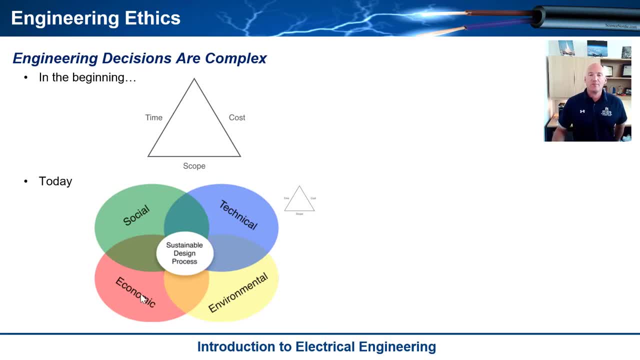 product right, It's not the phone, but it's like the economic impact of society. So when you're going to build this system, where is the system going to be manufactured right? And what's going to happen when you make that decision is that all of a sudden, there'll be an economic impact on. 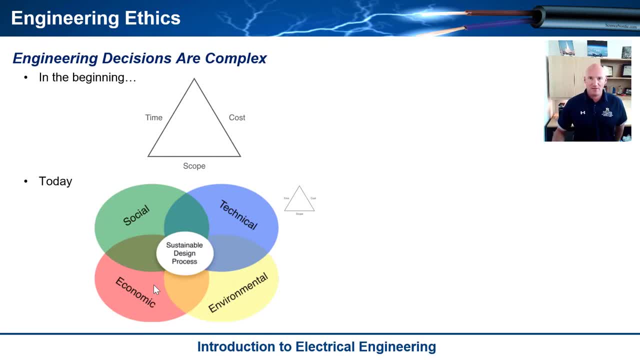 a certain area of the country due to, you know, the manufacturing, the manufacturing, and what is that going to do to the economy of that city? How is it going to change it? How is it going to be better? Or are you going to turn the city into an industrial district and stuff like that? So 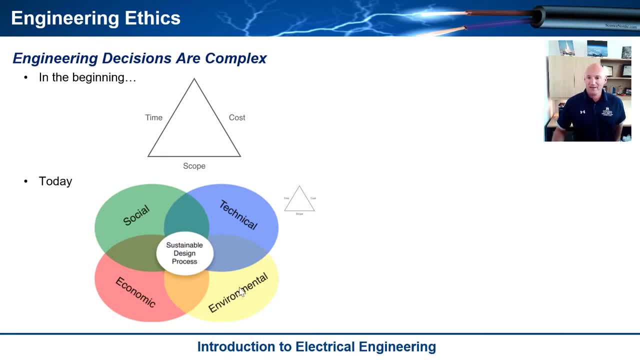 there's an economic variable here, And then there's the environmental impact, which is: you can't harm nature. You know, if you look at some of the solutions that we have right now from engineering, they harm nature, right. I mean, we're burning coal like crazy to boil water to make. 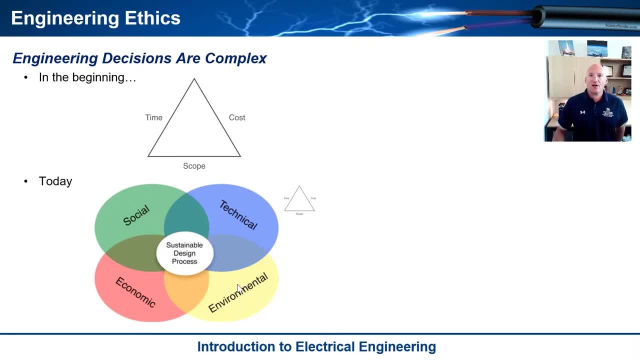 that's hurting the environment, And we just kind of thought, oh, the air will take care of all this smoke, And it's like now it's not taking care of it. We're producing too much, So you have this whole environmental impact of it, And so you got to make sure that your systems don't harm the. 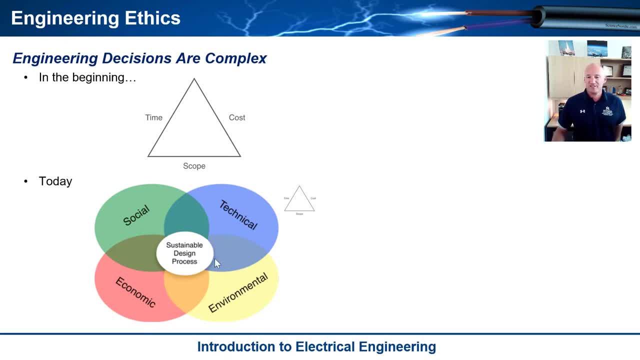 environment And then bringing all this together kind of, is this sustainable design process where you're no longer able to make design decisions that are just these open-ended? who knows what's going to happen after the system you know is done? It's like, no, you got to be able to sustain. 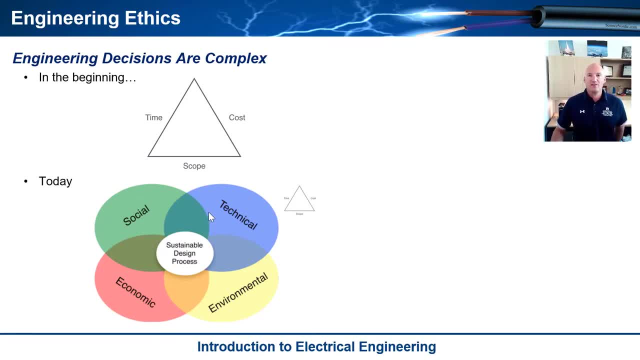 the system and then also obsolete it in a way that doesn't leave harm to both society, the economy and the environment. You know, and if you think about it like that, then you start thinking about. you know environmental is easy, right. It's like if you're going to build a copper mine. 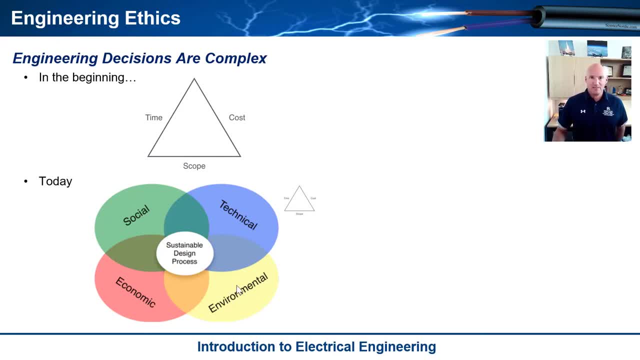 you can't dig a big hole in the ground and just walk away from it, right, So somebody has to fix that. But also, if you're going to build an economy for a particular city, what's going to happen when you decide to not? 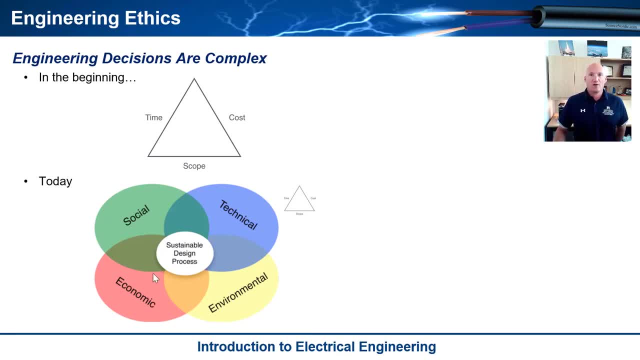 You can't have that manufacturing plant there. So you can't just walk away from a city and then all these jobs disappear and just you know, the whole city just collapses. So you have to. there's a lot of variables going on here and it's kind of challenging. So engineering decisions, it's a. 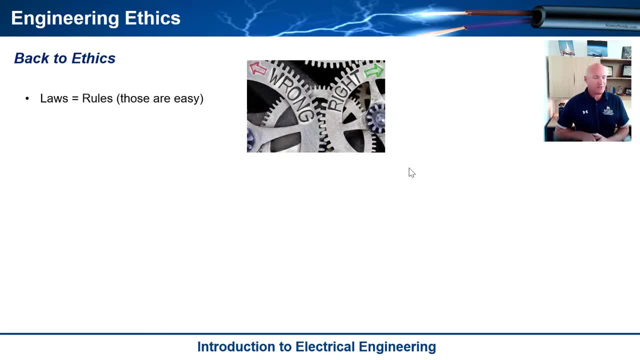 balancing act, And let's go back now to ethics. okay, So now, how are we going to do this? How are we going to balance all these decisions in the, or framed within the whole concept of making ethical right and wrong decisions? Well, let's think through this a little bit and see how it can become very an interesting even more. 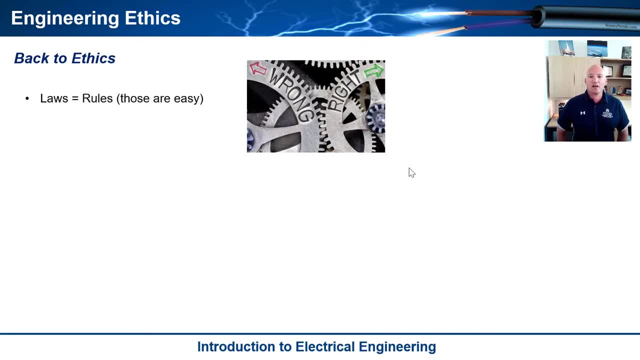 interesting challenge. So, first of all, when you think about ethics, we're not talking about laws, okay, So everybody understands: if there's a law and you break it, it's illegal. And even when you have different countries that have different laws, they're easy to follow, right, You find them. 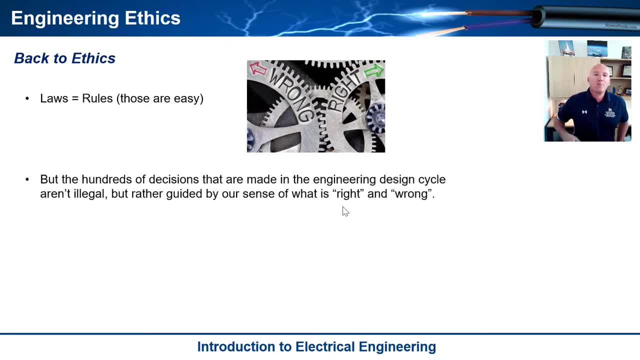 you don't break them okay. So those are actually kind of easy. So when you talk about ethics and how it impacts engineering decisions, what we're really talking about is, you know the hundreds that you make in a day, the hundred actions that you take in a week that guide your whole design. 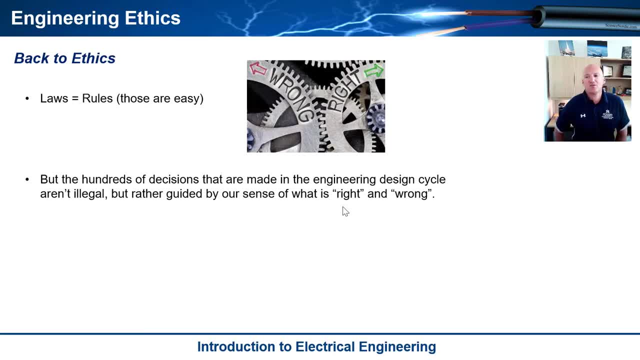 philosophy or your design process, okay, And so these, these decisions aren't illegal. right, These are all legal things, but it's just kind of like how, how do you make those decisions and what kind of influences you? And this really comes down to it's usually a culture, right, So it's a culture. 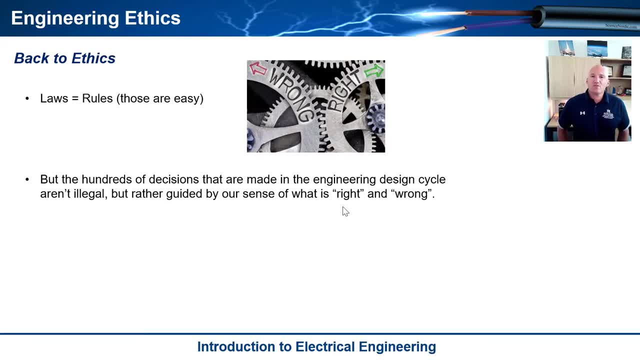 of you know the business that you work for, And it's also a combination of your own moral code, right? I mean, it's it's your background that brought you to this this time and place, And so here let's look at a 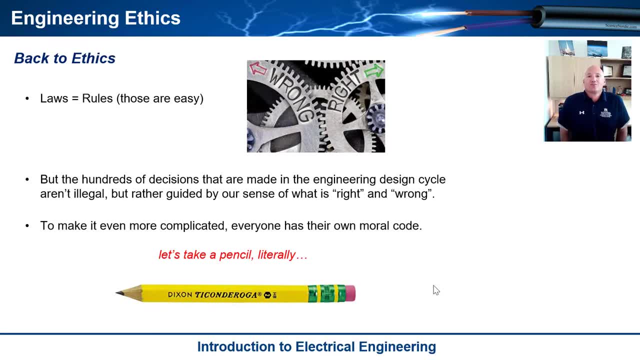 really simple, kind of a silly example to kind of illustrate this point. And so let's, let's think about a pencil at work. So you get a job for a company and they- you're an employees- they're going to provide you everything that you need to to be successful at your job. So that's a desk. 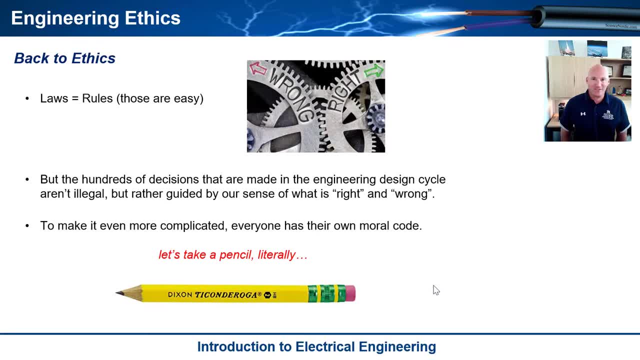 and a computer and a chair, and paper and pencil and staplers and everything. So you have all this stuff that you need to be successful at your job, right, And so what you're going to do is you're going to take a pencil from the supply cabinet and take it home, Okay, And the knee jerk reaction that 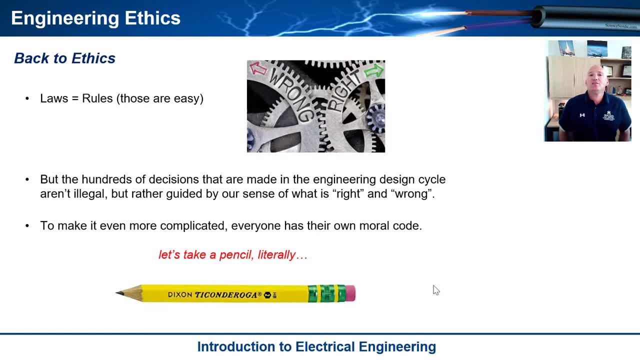 most people have is: no, that's stealing. And then you sit and you think about it, just not even for five seconds, And all of a sudden people will start realizing that there's more to it. right, It's like, well, wait a minute. What you know, I do work at home. right, It's like I'm a salaried. 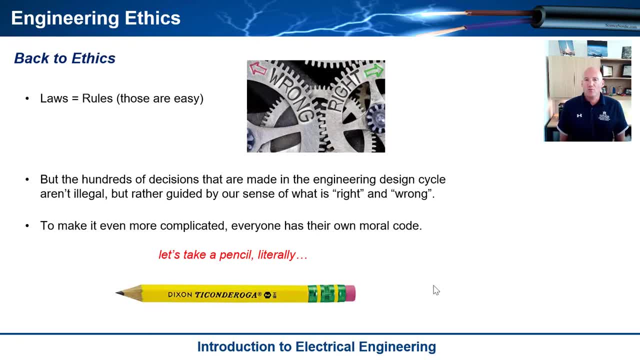 employee I'm. I'm always kind of working, So when I'm at home, if I'm working for on stuff that's for that company, shouldn't I be able to use that pencil at home, because I do write down notes and everything? 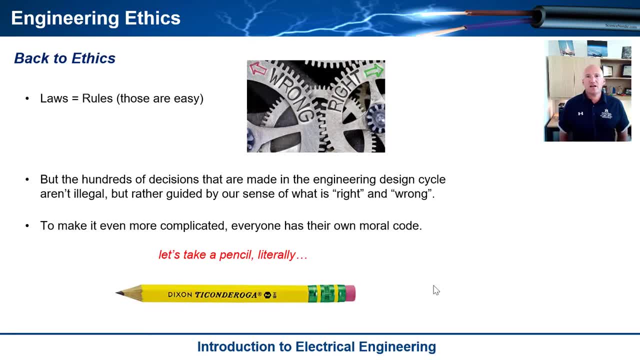 And it's like: well, yeah, So then you can kind of convince yourself that it's like: yeah, it is, it is okay to take that pencil home, And yeah, you might use it for personal use too, but it's, it's. 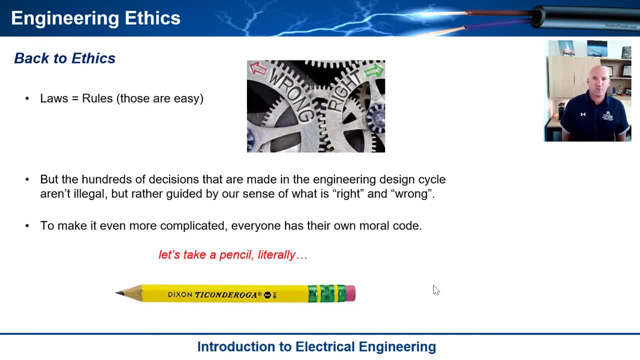 it's kind of silly to, it's a waste of your time to like have a pencil at home that's for your personal and then you have a work pencil and stuff like that, And so even something as simple as a as a pencil kind of illustrates that there's this, this gray line of like it's not really right And 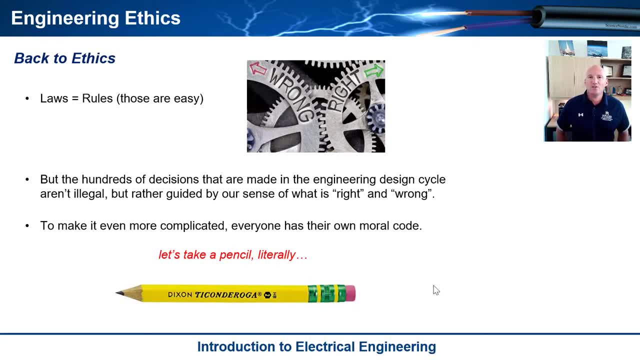 it's not really wrong And it's not illegal. but how do you? you know it's what makes you make those decisions, You know it's what's your background that gives you that you know decision making ability. And then if, then, if you. 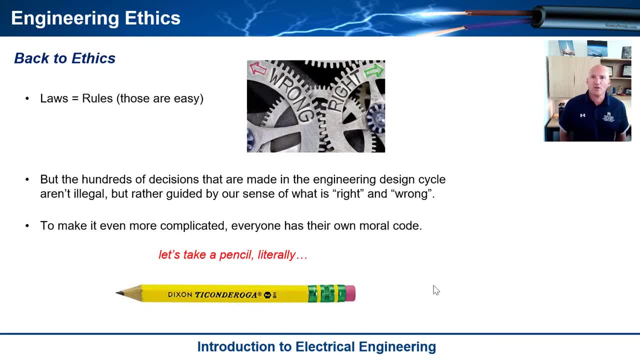 kind of go back to the knee jerk reaction of like no, it's illegal, then you might go. well, why don't if? if it's gray zone, why don't we just make a rule? right, Let's make a law or a rule. 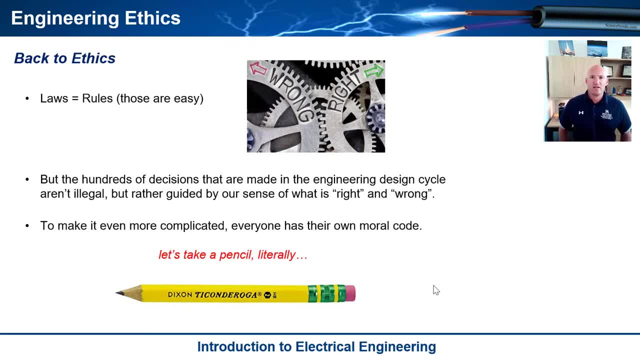 within the company that you cannot take home a pencil. Okay, Let's, let's just make it really clear so that engineers don't have to worry about that. Right, these gray decisions. Well, if you expand that, what you realize is that you would have to have 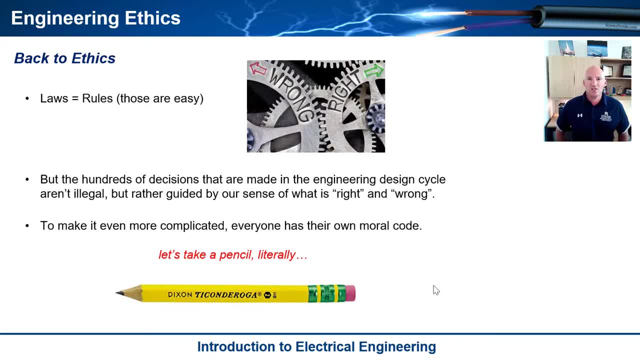 a rule for almost every single situation that may ever arise, And there's so many rules that would be needed to govern all the thousands of actions that you take each year and every decision you make that it becomes impractical or it is impossible to make rules for every situation. 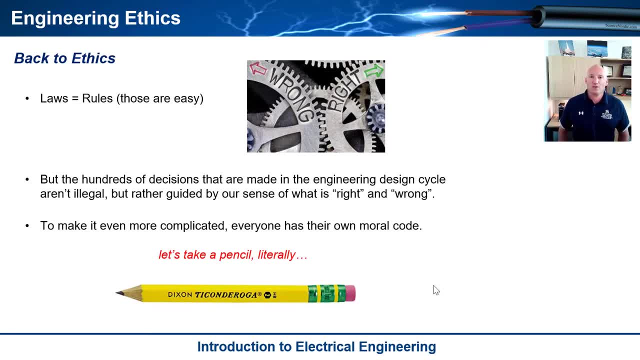 And so this now is kind of this ethical framework that we live in And a lot of people will call it like micro ethical decisions. So it's not really like you get faced with this thing where it's like you need to design. your boss tells you you need to design this and it's going to kill people and 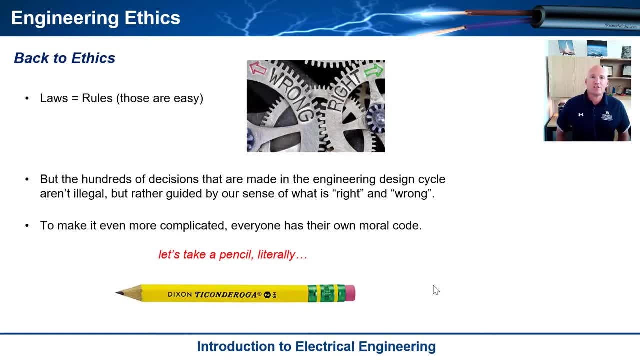 you need to do it because we're going to make a lot of money, right? Those aren't the type of situations that we're faced with. It's these just hundreds of very minor situations where you tend to favor one direction versus the other, And it's because of a culture, potentially at your workplace. 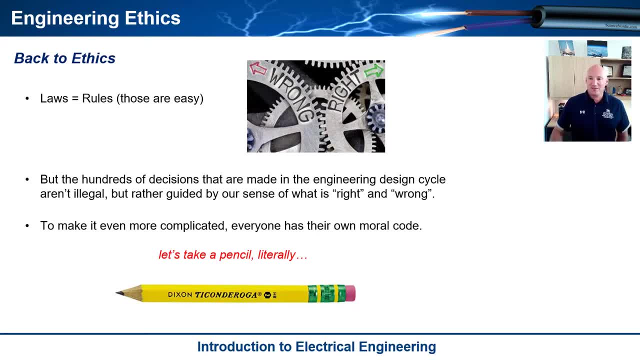 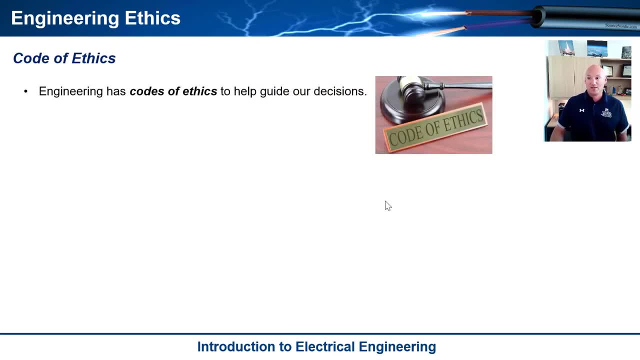 Okay, So I think that's a really good point. So I think that's a really good point. So this is- yeah, I know it sounds scary, but it's like this is just the motivation for why this is a complex and very important subject. Okay, So you know, it's like I can't do this right. I mean, I'm learning. 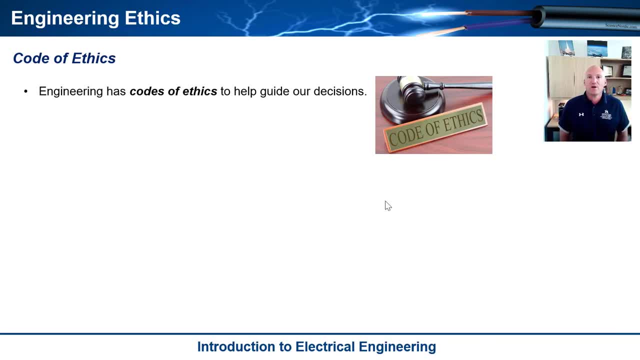 electrical engineering. It's taken me four or five years to get through the bachelor's degree. I can barely make it through all this complex math. And now you're telling me, oh, and, by the way, you also need to be a philosopher. Okay, And you also have to have you know, understand morality, like every. 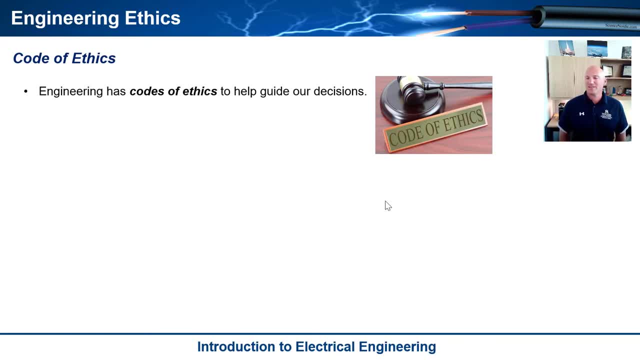 philosopher has ever understood it since the beginning of humanity. It's like: okay, no, no, no, no, no. This is something where you use knowledge from other fields to help guide you, You work with other people from other fields to help guide you, And we have also come up with tools and techniques. 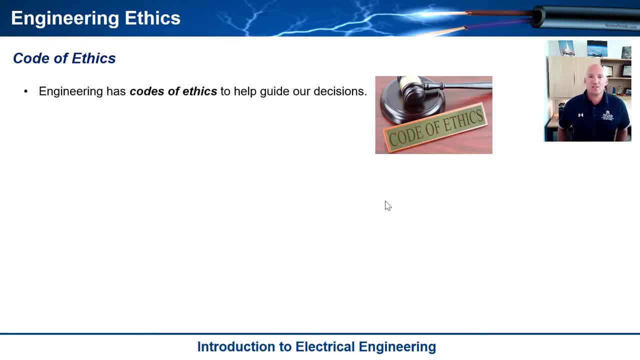 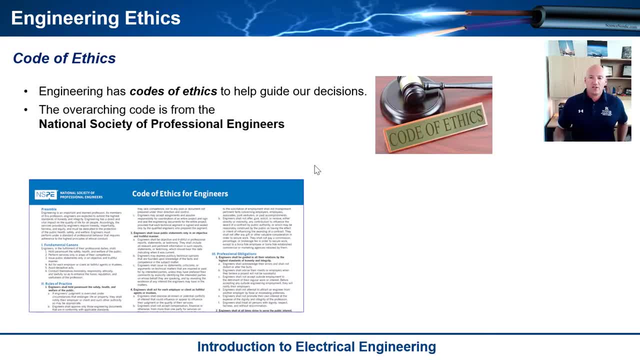 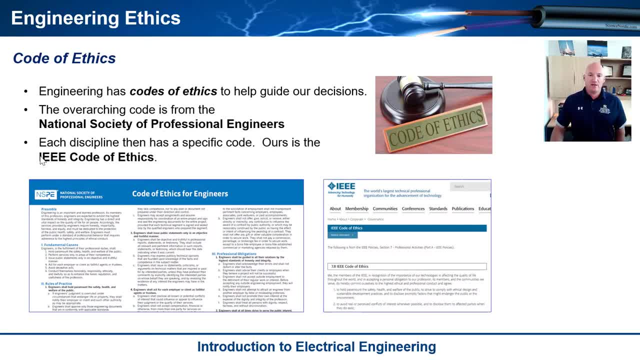 you would expect, Within electrical engineering, we actually have a professional society. It's called the International the Institute of Electrical and Electronic Engineers, IEEE, And it has its own specific code of ethics. IEEE happens to be the largest professional society in the world, And so they felt like they had to come up with their own code of ethics, even though 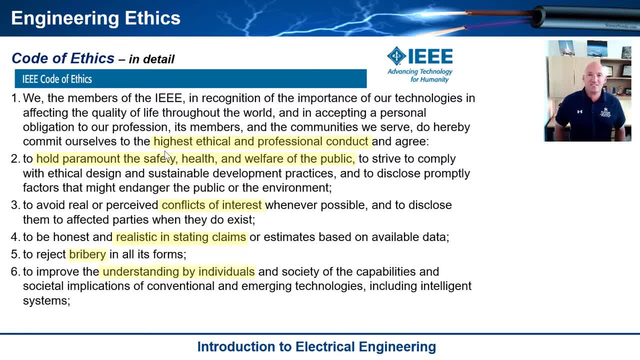 it's very similar to the other ones, But just to go through it there's there's like 11 steps And it really is common sense. It's stuff that you would think anyway, But it's, it's if you write. 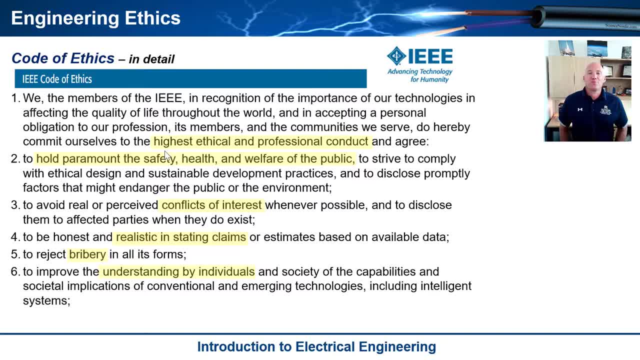 it down and say: and everybody agrees that this is what we're going to do, then it kind of provides, like this mini law book for you that you can always consult with. Okay, So really quick, let's just go through some of the highlights of it. So you know, we are going to hold ourselves to the highest. 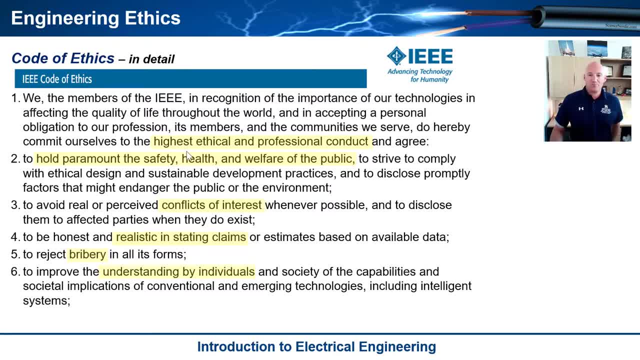 ethical and professional conduct By agreeing to the following: we will always hold safety and health of the public paramount. We will always avoid conflict of interests. We will be realistic in stating claims. We will reject bribery. We will under. we'll improve the understanding of individuals. We'll try to educate our stakeholders. 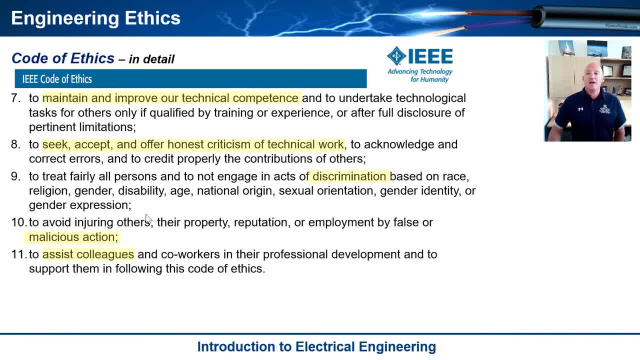 so they understand what we're talking about. Okay, We'll maintain our own technical competence. So it's it's not okay to just get a bachelor's degree and then say I know everything in the world about electrical engineering. You have to continually improve yourself as technology changes. You have to look, you have to get. 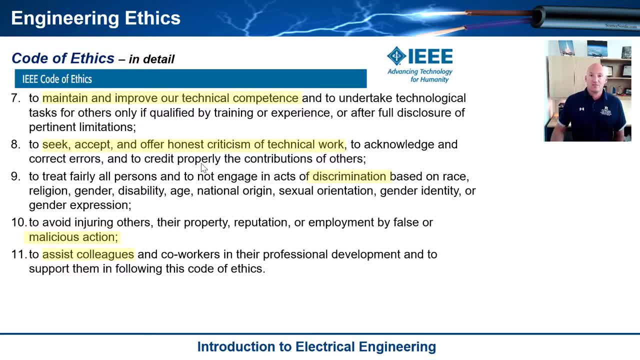 peer review of your designs. So get honest criticism of your own decisions. You don't engage in discrimination against anybody. You don't have to do malicious actions to injure other people or, you know, injure their reputation, And we also agree to assist each other in their own, in our own. 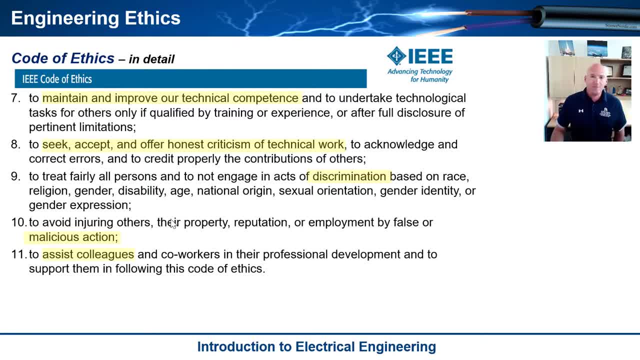 professional development. So we're in our, in other people's designs. Okay, Pretty, pretty, pretty common sense. This is almost like you know, don't murder people, right? Everybody agrees. And you think, why would you have to ever write that down? It seems common sense. Well, it's pretty powerful to have. 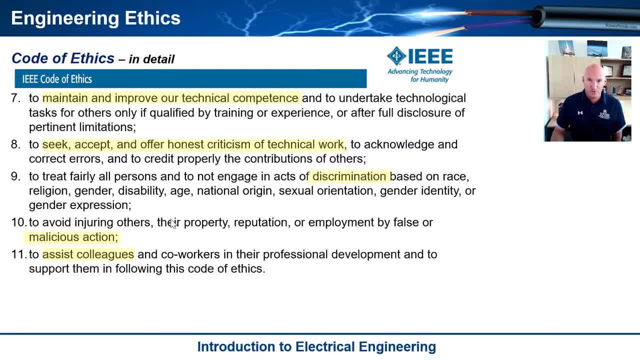 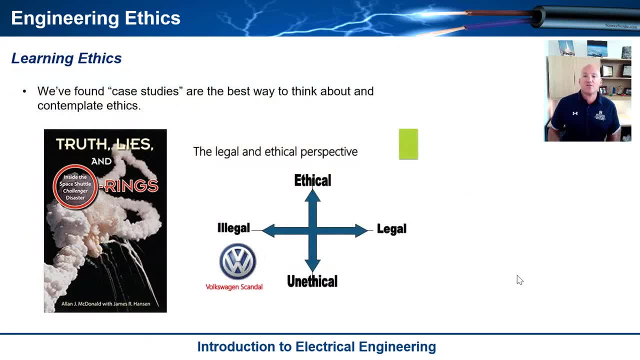 something written down, because it gives you something that you can refer to when you're faced with situations, And you can always come back to this and say, Hey, the code of ethics helps guide me. Okay, So that's the first thing that you know engineers get exposed to when it comes to ethics. 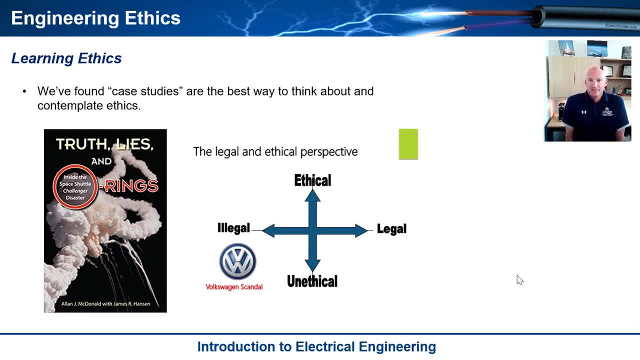 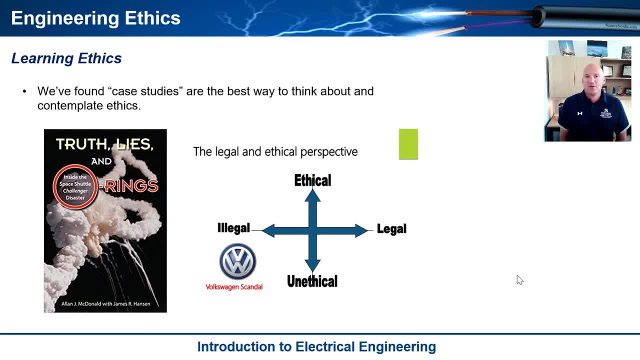 pursuing a degree in electrical engineering and you're learning about circuits and all this stuff. then you have kind of this whole ethics thing And and we also, we have this notion that there's there's like no right or wrong, right, Correct, And it's. it's kind of true, right, So it's all. 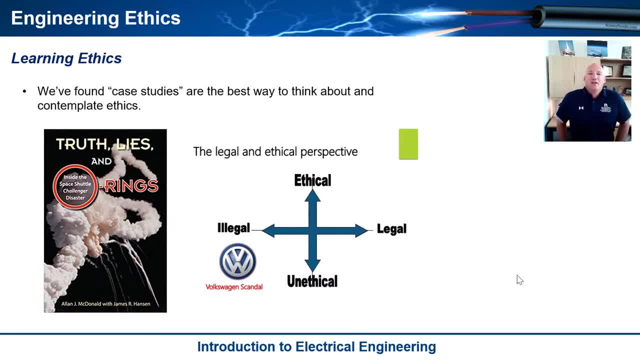 these little micro ethical decisions that people make that compound on themselves. So what we've learned is that the best way to understand ethics and to learn about it is by case studies, And so when you take classes in in ethics, you can talk about moral frameworks and decision-making frameworks. 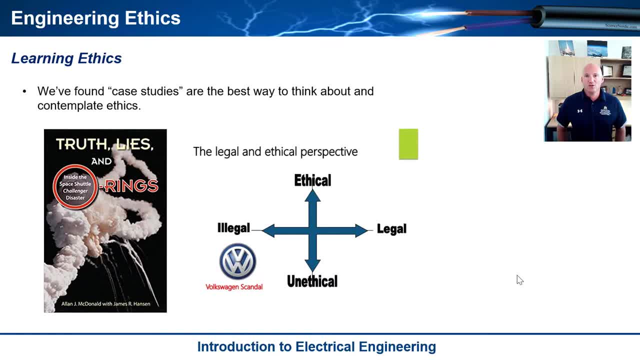 and how they integrate. But really, what you like to do about when you learn ethics is you look at other situations that people have been into or have been in that resulted in some problem. Okay, So you know, a classic one is like the the space shuttle challenger, where the O-rings caused it to 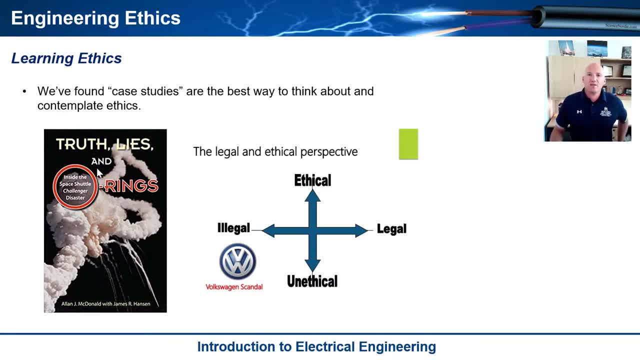 explode. And so when you there's books and books written about this and what you see in it is that it wasn't like this, this one moment, right, It was just a series of decisions and in a culture that kind of swayed certain decisions from being made or voiced, And it was a whole lot of small. 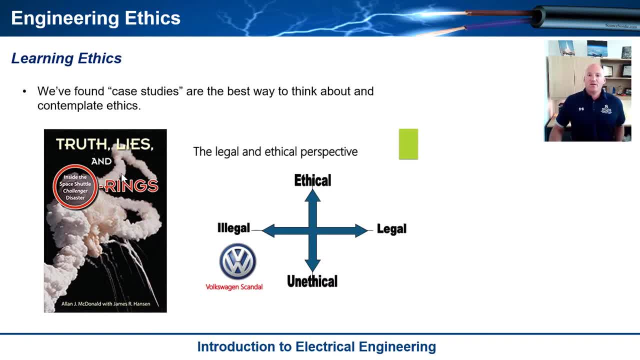 things that ultimately led to a catastrophe, And so it's. and when you look at that, you can kind of look at patterns that emerged and and understand it's like, well, yeah, I, I can see it happening. right, There wasn't one moment, but you can see the patterns that happen And 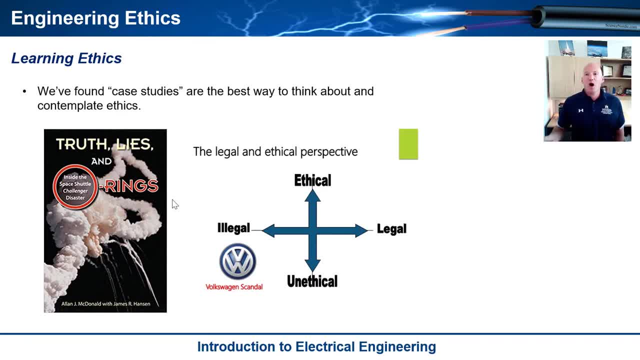 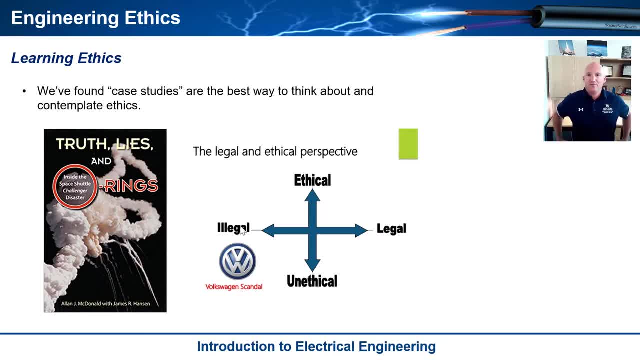 cultures. Another one is like the Volkswagen scandal. So this is where they- you know Volkswagen- actually built software into their, into their cars, So that when they did emissions testing it would know it's being tested and it would put the car into a low emissions mode. 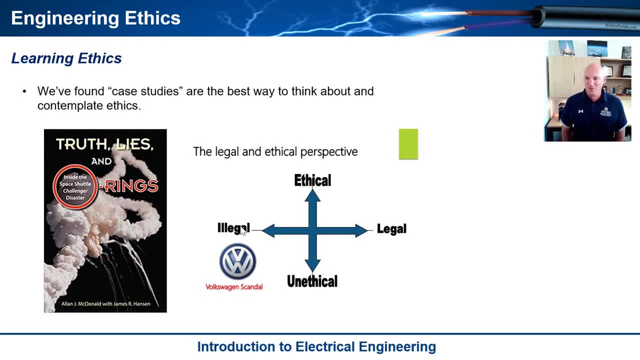 And then as soon as it got out of the test, it would crank back up and put out more pollution. And so you think like there it's like wow, that is just flat illegal, Like that was breaking the law. But again, 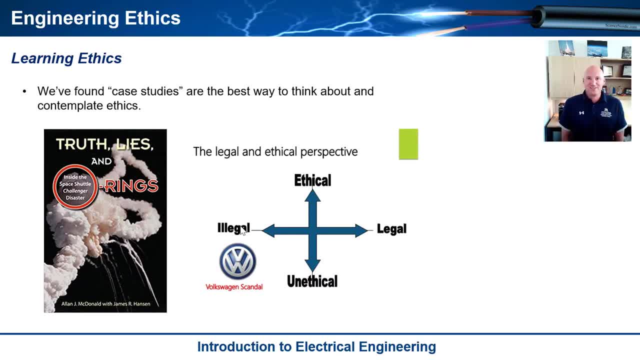 it wasn't like there was one evil business person in the company that just says I am going to make this happen. It was a whole lot of things and a lot of different people that were. this culture kind of shifted the balance of decision-making toward a kind of toward an end end result. that 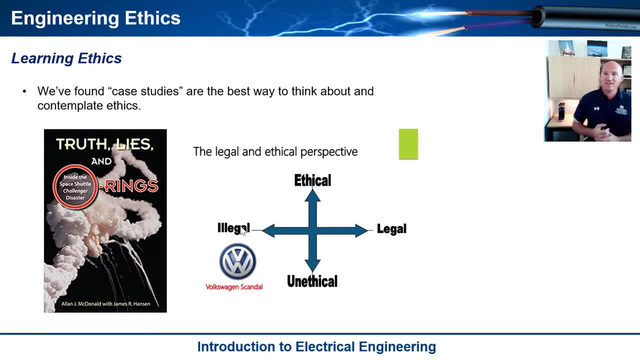 ended up being illegal. And so by looking at that, you can start identifying these patterns earlier and understand, like when these just understand, like how these things actually happen, Because when you hear about them it just like a really quick, you know really quickly. you're like: I can't. 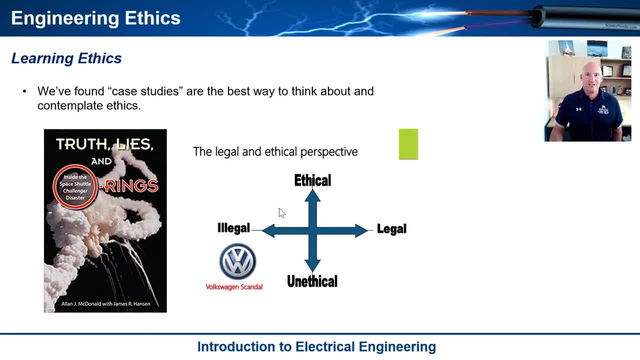 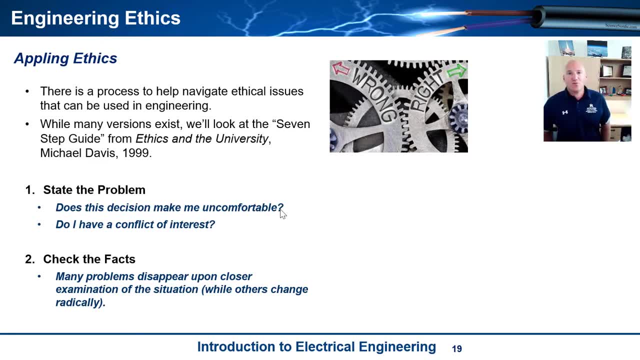 believe that happened, But it's only when you really study the whole, the whole process and the history of it, that you start seeing these patterns. Okay, finally, we get down to applying ethics. So once we've you know we've talked about why engineers are important to society, why our 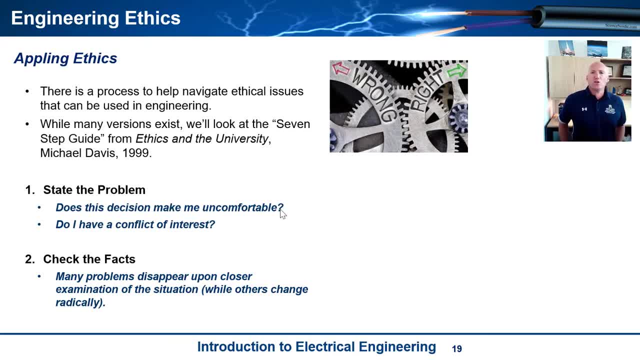 ethical decision-making is important. We have a law. you know, we have the laws, we have the code of ethics, We have all this stuff. We learn about it using case studies And finally you get to be an engineer and you get to practice this and you get to apply ethics. So it turns out that we have a 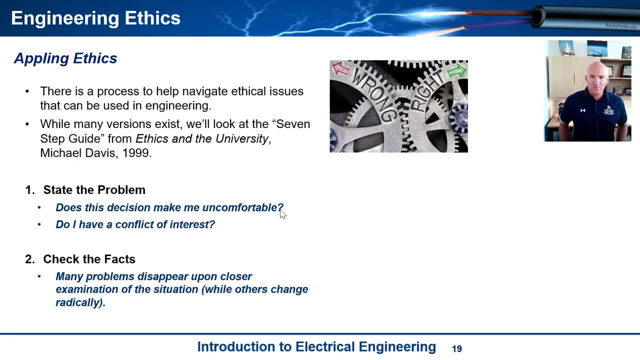 step-by-step guide that helps us apply ethics, And there's there's different versions of it, but I'm going to give you, I'm going to show you one that's called the seven-step guide from ethics and the university by Michael Davis 1998.. And it helps us navigate these ethical issues that come. 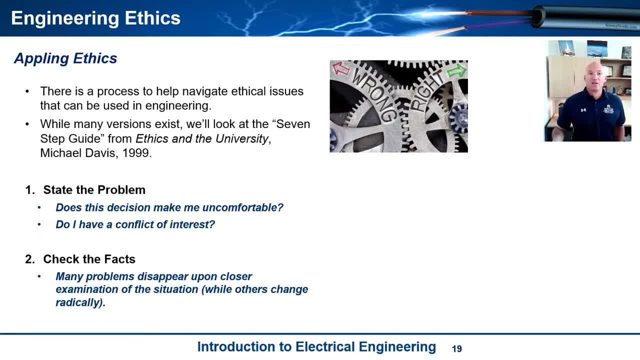 in engineering. And this is just one application of one version of this application, but it'll, it'll kind of show you that it's not just you're not just alone, right, You're not just like. I hope I make the 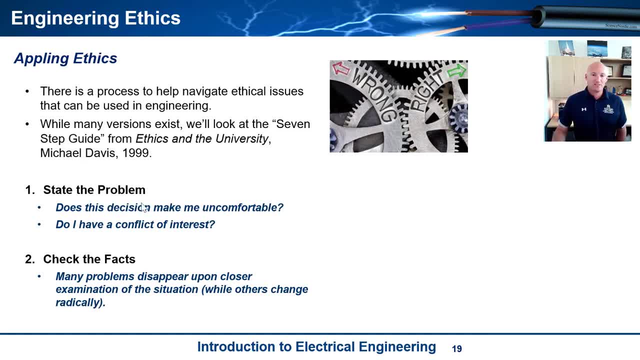 right decision. It's like: no, no, no, no, this isn't. we're going to apply a process to this. So step one is, if you are faced with something that doesn't feel right, you state the problem. Okay, why does this make me? 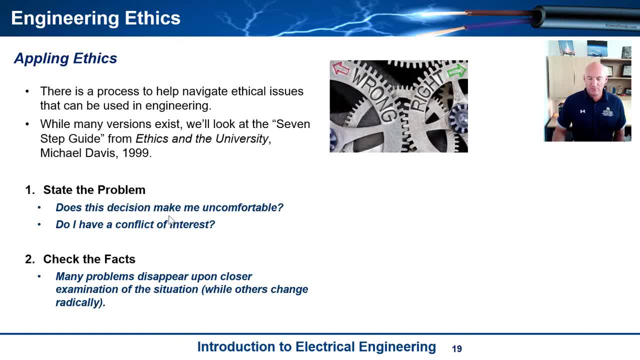 uncomfortable. And do I have a conflict of interest that's making me feel uncomfortable? You should never feel uncomfortable as an engineer. Okay, if you were working at a place and you're, you're uncomfortable with something that is not normal. Okay, you need to stop and go. 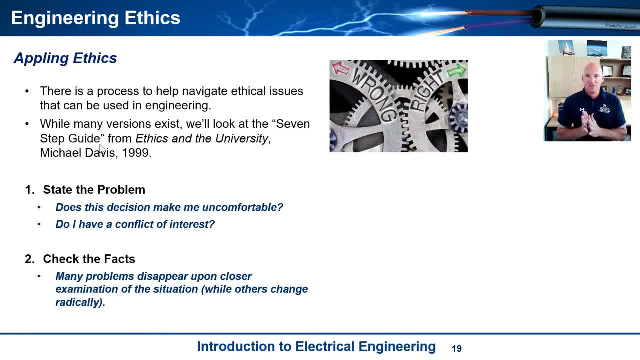 what has happened. Why do I feel so uncomfortable about this situation? Engineering is not. it's supposed to be fun, right? I mean, you're really doing some important works, so it's not supposed to be uncomfortable. So if you ever feel uncomfortable, you got to stop and just say: 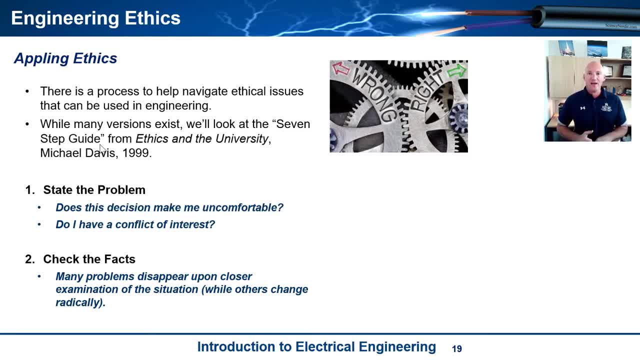 what is going on here And you state it, you write it down and say: why is this problem making me uncomfortable? And so that right there allows you to say I might have an ethical situation. The next thing you do is check the facts. Okay, A lot of times you people, a lot of times people. 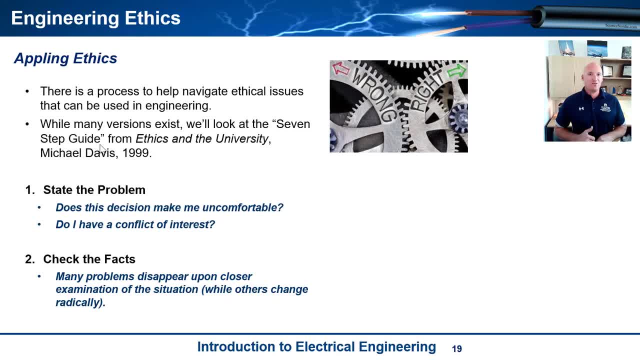 don't have all the information, And if you don't have all the information, sometimes you don't see the big picture. So the next step that you do, number two, is you get more data. So you check all the facts and try to get the background, And almost always, once you have a situation that 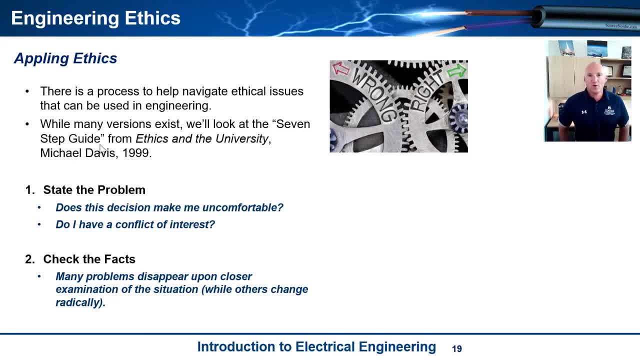 makes you feel uncomfortable. if you're able to get a bigger picture and more information about what's happening, most of the times you realize that it's not an issue and you don't feel uncomfortable anymore and you're able to proceed. However, if you don't, 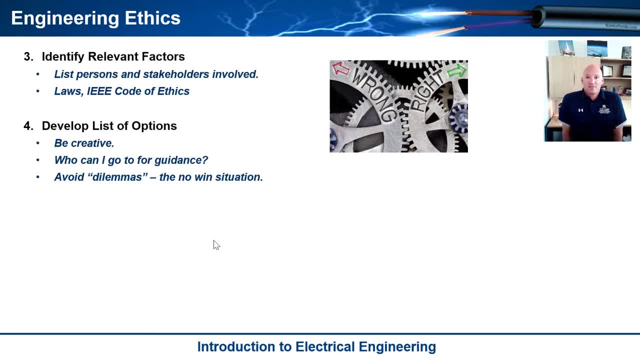 you need to do is say I might have something going on here. that's an ethical dilemma. And the next step, number three, is you need to identify relevant factors. So you're going to sit here and you're going to go. I'm going to list the people and the stakeholders involved And I'm 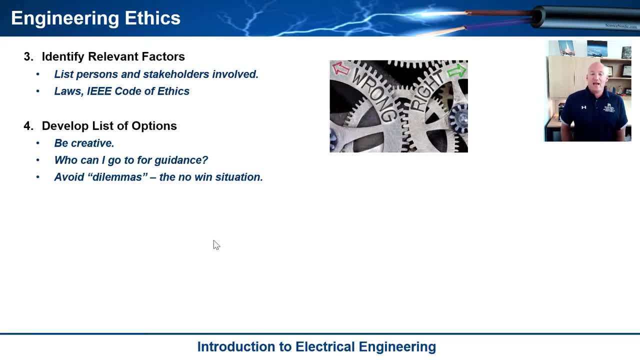 going to look at the code of ethics and I'm going to look at these things and I'm going to start thinking about: okay, are we really violating the code of ethics? Okay, Who might be doing it if it's not you? And are there people that might have a problem with it? And I'm going to look at these. 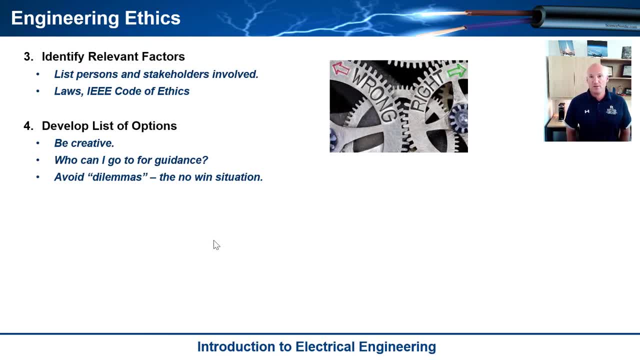 and I'm going to start thinking about conflict of interest. that would be leading them to violate one of the code of ethics statements. Okay, So then once you get that down now you kind of have more you know, have it like a case for what's happening. Then you problem solve. So number one: 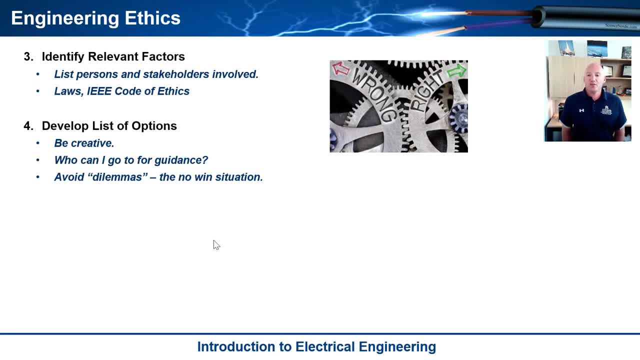 develop a list of options. Okay, First of all, avoid dilemmas where you have no win situation. Every situation is a winner. Okay, So you got to have solutions and be creative. Okay, So it's like: who do you, who can you go to for guidance? You know, seek mentoring on what to do. 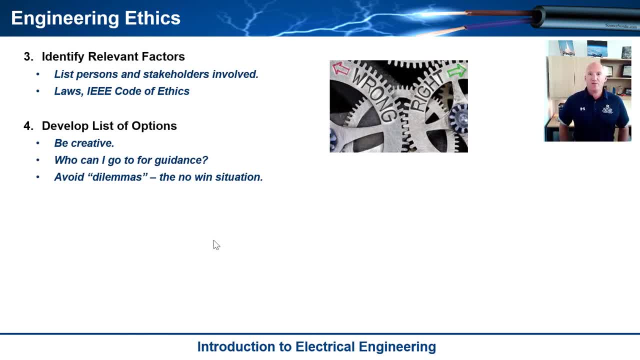 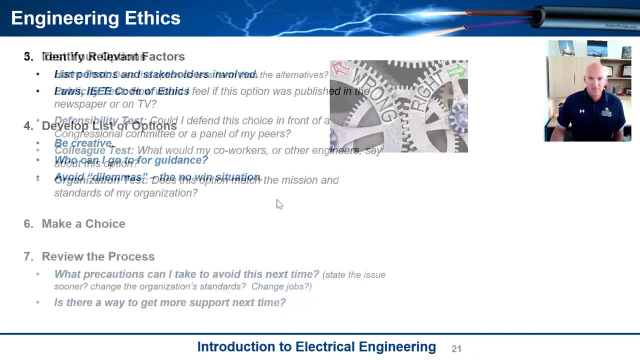 come up with different ideas on how you could resolve this without it being just a horrible situation where there's no way out, And then, now that you have solutions, you can start proposing them. Okay, Okay, Then what you got to do is take these tests, So we call testing our options. 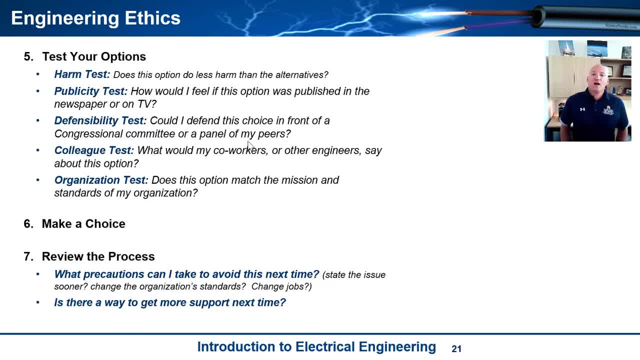 Okay. So, as you think about how to proceed, there are a variety of different tests that have been developed by people that allow you to see if these ethical situations are real and if your solution is good. And so there's the harm test, the publicity test, the defensibility test. the colleague 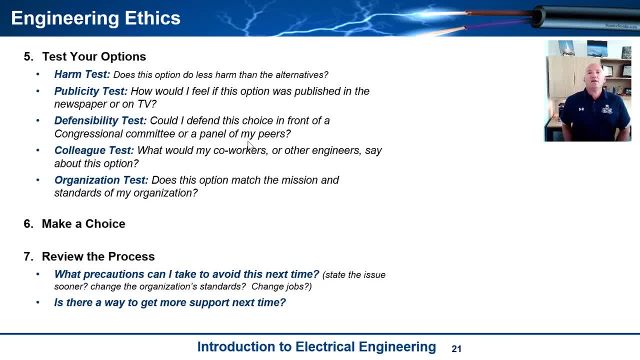 test and the organizational test, And these are. these are things that you apply personally, based on your own background. So the harm test, for example, is: does this option do less harm than the alternatives? Okay, And so your solution you've come up with. is it better or is it actually? 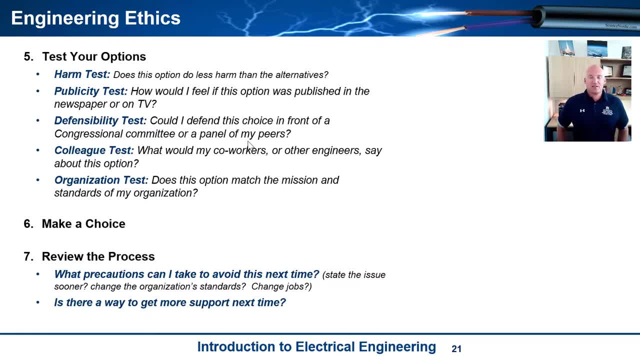 worse. The next thing is the publicity test, And this is interesting. So if you pursue one of your options, how would it make you feel if it was published in the newspaper or the TV, So the general population saw this? Would you be able to see if it was published in the newspaper or the? 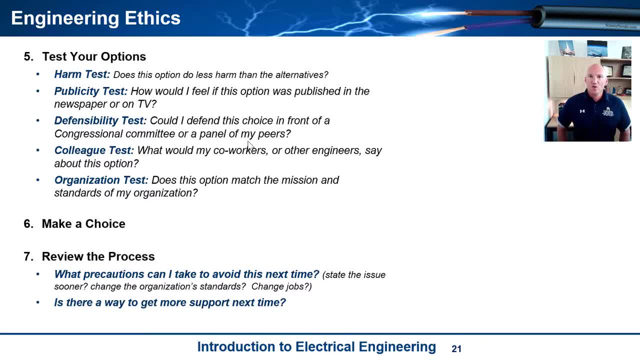 TV, Would you be embarrassed? Okay, So if your, if your family saw this, would you be like, wow, I can't believe that I did this. I can't believe I pursued an option that was a solution to this issue, or let the issue proceed. And my family looks at me and they're very disappointed. How? 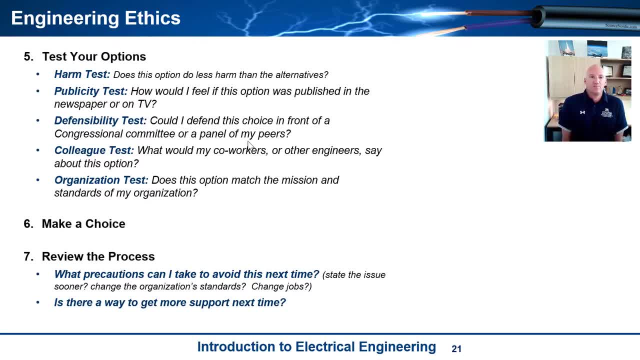 would that make you feel? If you're willing, if you're able to have this be publicized, like on the front page of the newspaper or on a, you know, on on TV, if you feel okay, then that's good, Okay, That's a good thing, Cause that's it takes a lot to be able to say that The other one. 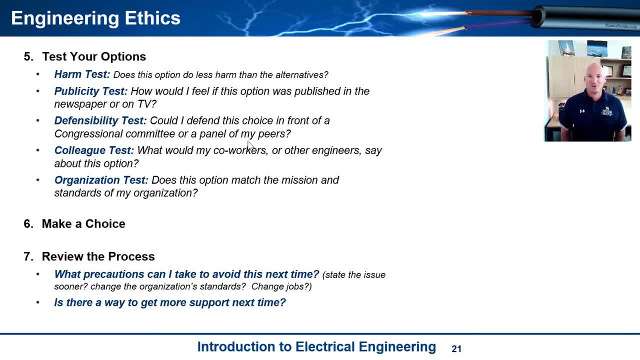 is a defensibility test. So let's say you got called before Congress or called before a judge and they said: you need to defend this action. Actually, it'd be probably more like Congress, but you need to defend this action. Could you actually defend it with logic? Okay, Could you? 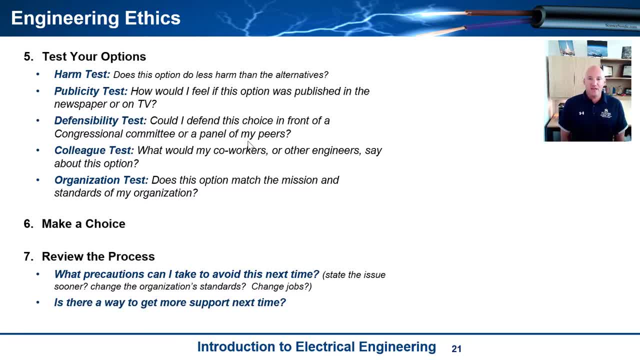 actually show why, why you came to this decision, and defend what ultimately happened. The other one is the colleague test. So what? what would your coworkers or other engineers say about your option? Okay, What you ended up doing? Would these peers 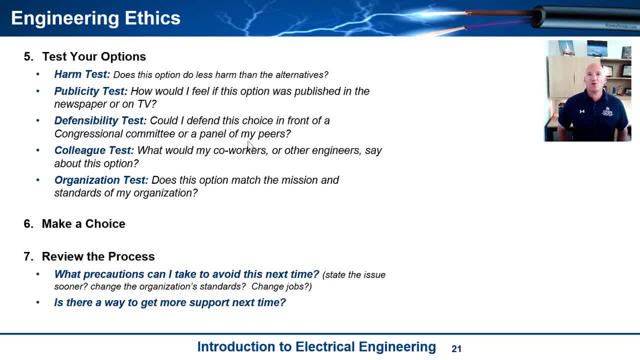 that have the same training as you? would they understand it? Or are you doing something, pursuing an option that is just so random that they would be like, wow, this is no good. I mean, this is, this is horrible, And then this is, this is the other one is: does this? 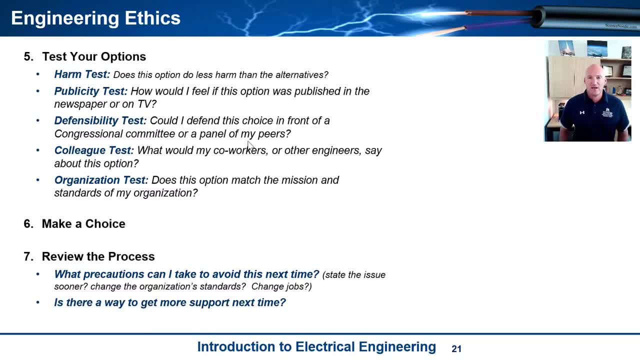 option. make the match the mission of the standards of my organization. Otherwise, other another way of saying this is the culture of the organization. Is this decision in line with the culture of my organization? Okay, And then you got to make a choice, Okay, So if you 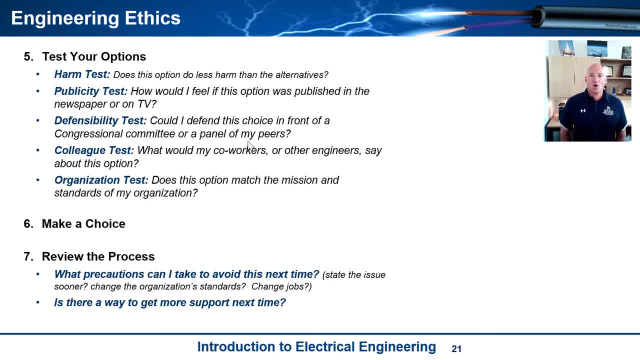 are in a situation where you're going to, you recognize something's wrong and you are going to propose a solution and let's say that it doesn't work And so it's rejected, and you know you're going down a path you have to make. 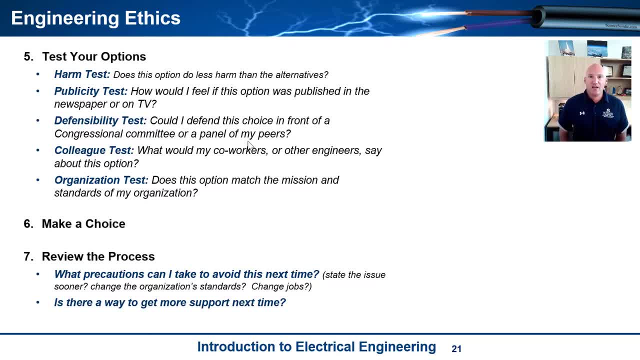 a choice. Your choices basically are: are you going to stay in the fight, knowing that you're going to be forced to do something wrong, Or are you going to pull the rip cord and bow out? We have laws called the whistleblower law that allows you to basically make accepting making a claim. 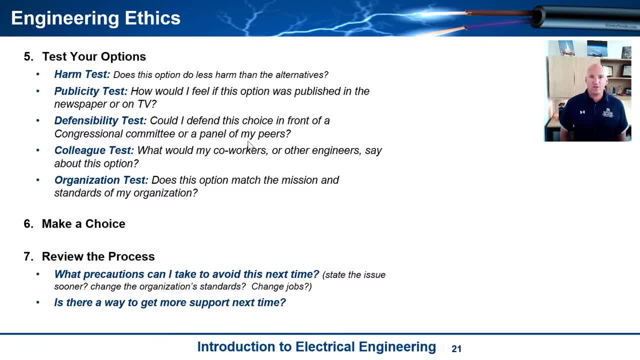 your organization without repercussions, and so you can always quit your job and file, or you don't even have to quit, you can. also, you can always file a whistleblower claim and you remain anonymous. but you need to make a choice at some point, okay, and then, finally, the last one is: uh, what review the 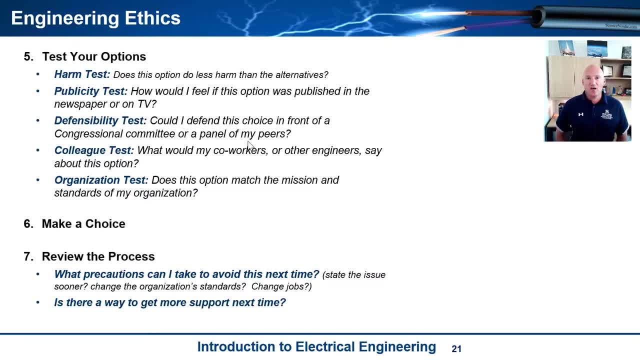 process. what precautions can i take to avoid this next time? so you're not done with engineering as soon as you resolve an ethical situation. you're an engineer for your whole career. so what can you do? what? what choices can you personally do to change an organization you're in, to choose an? 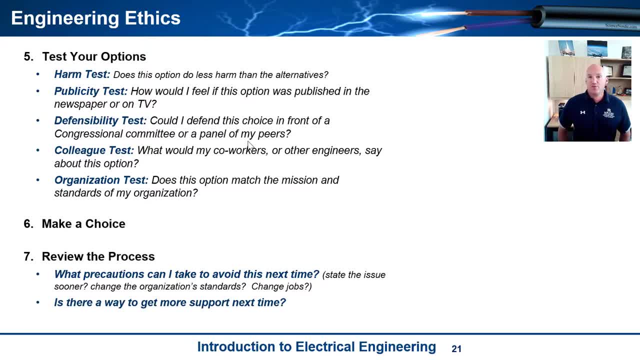 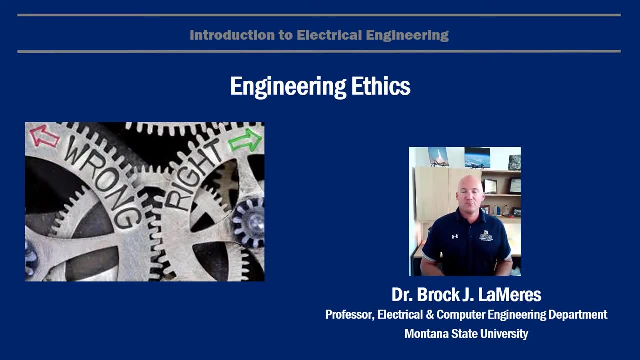 organization, uh, that you want to be part of, to maybe influence laws, uh. and then there's: is there a way to get more support for yourself next time? okay, so this is. this is pretty complicated stuff, right, but there is a process. it's not just you alone where you have to make some really. 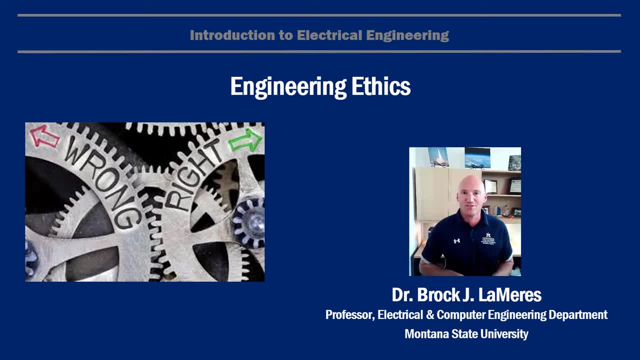 you know, very difficult. more morality choice. uh, there are the code of ethics, there are processes, there's a whole system of framework on how to learn about how to do this stuff and how to recognize situations, and so that is an introduction to engineering ethics. hopefully it kind of 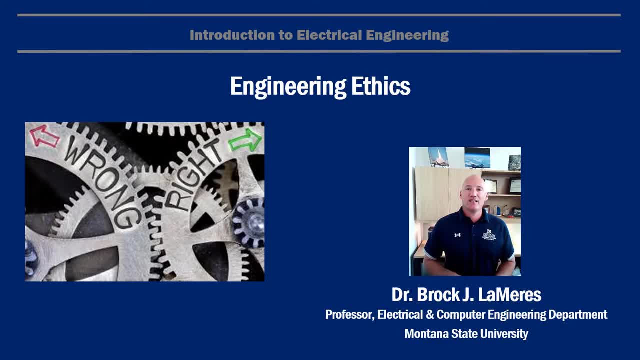 motivates the need for this and it will kind of explain why you're going to see so much of it as you continue to study electrical engineering. all right, that is it, and we'll see you.